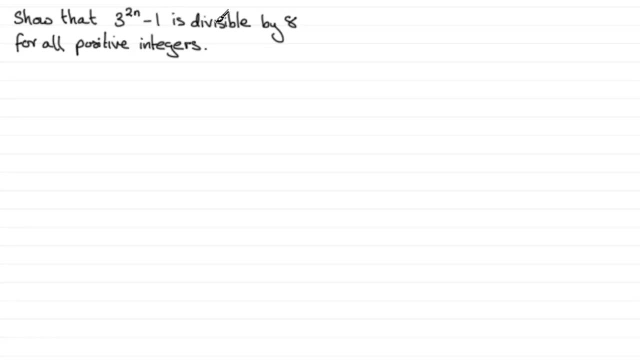 show that 3 to the power, 2n minus 1, is a multiple of 8 for all positive integers. It's the same kind of proof that we're going to use. So what is this proof? Well, like all induction problems, we have to. 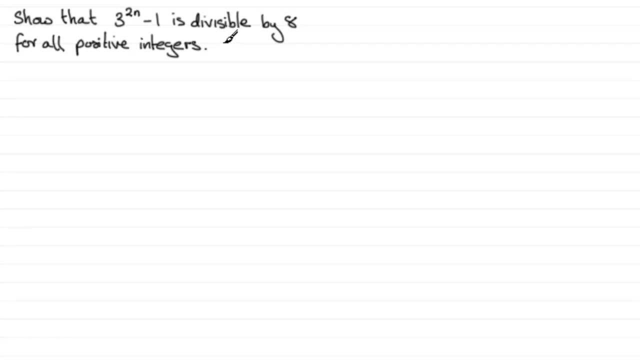 show that it's true when n equals 1. Then we assume it's true when n equals 1. Then we assume it's true for n equals some value. say k, and go on to prove that it's true for n equals k plus 1.. And on that, 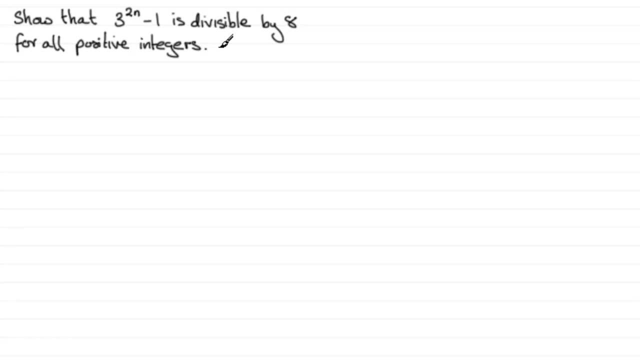 basis. if it's true for n equals 1, it'll be true for n equals 2, 3, 4 and so on. But when we're doing these divisibility tests, we have to handle them in slightly different way to what we've done. 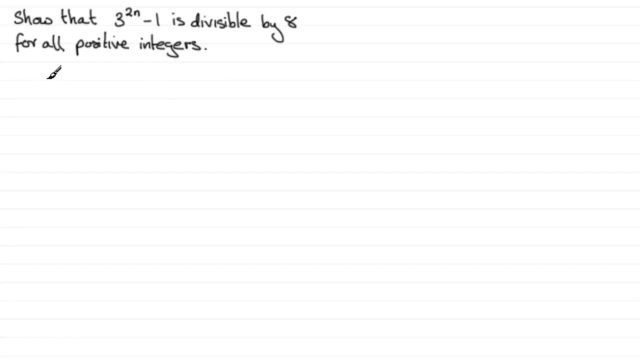 before. I'll show you What we tend to do is define a function. In this case let's say f of n, be that function which is equal to the expression you've got here, So 3 to the power, 2n minus the 1.. So we need to check out first of all that it holds when n equals. 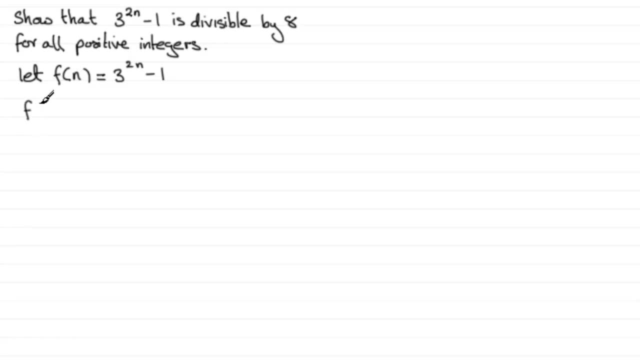 1.. So we'll just say f of 1.. What does it equal? It's going to equal 3 to the power, 2 minus 1.. So we're going to check out first of all that it holds when n equals 1.. So we'll just say: 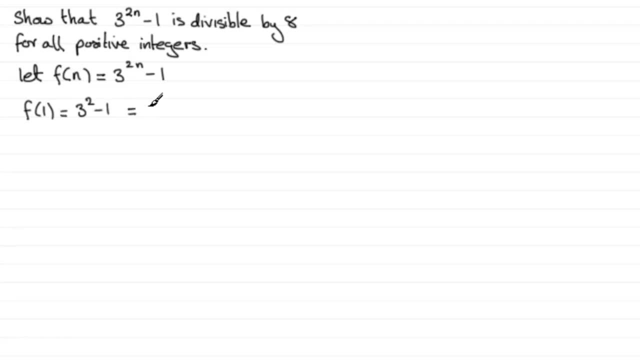 f of 1 minus 1.. In other words, 9 minus 1, which equals 8.. So clearly, f of 1. when n equals 1, it's divisible by 8.. So we can say therefore: true, when n equals 1.. Now we go on to assume that it's. 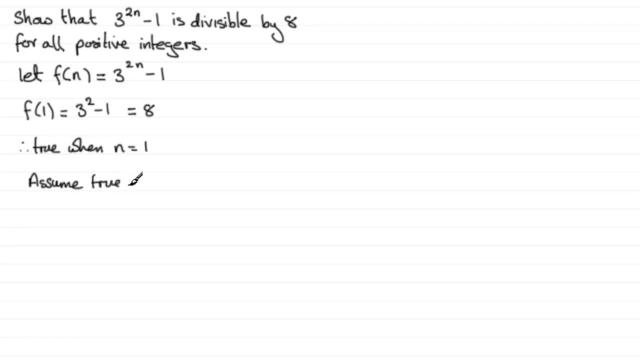 true. Okay, we'll just say: assume true, for n equals some positive value. So we're going to say it is k. So we know that, therefore, f of k, which will be equal to 3, to the power 2k minus 1.. 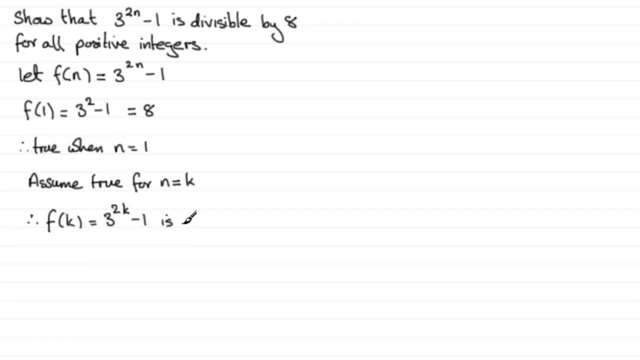 We know that that, or assume it's divisible by 8.. Okay, divisible by 8.. Now, on this basis, we are going to show that this is going to be divisible by 8.. Now, I said this was slightly different to what we've done in the past. When we're doing these divisibility tests or multiple tests, what we 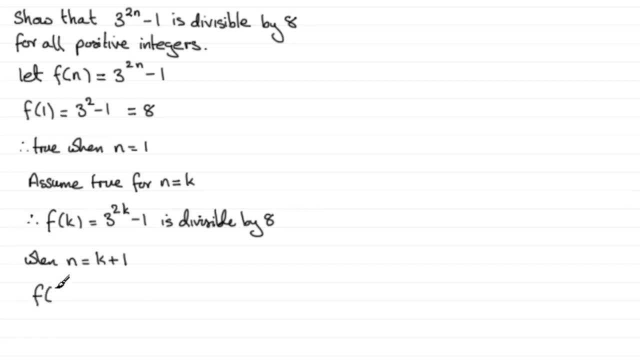 always look at, is f of k plus 1 minus f of k. All right, And what I'm going to do now is substitute for what f of k plus 1 would be, So that would be replacing the n here then with k plus 1.. So we're going to get 3 to the power 2, lots of k plus 1. 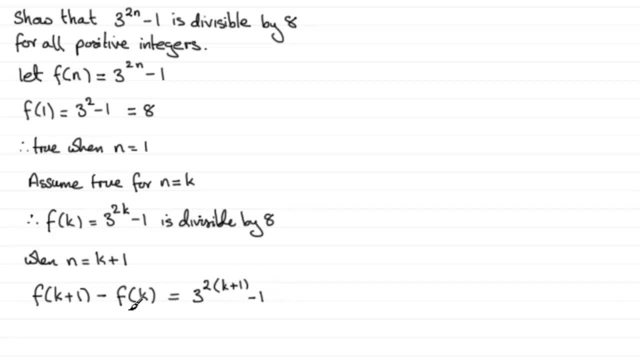 and then that's minus 1, and then we've got minus f of k, So that's going to be minus 3 to the 2k, minus 1.. So I'll put that in brackets though: Minus 3 to the power 2k. 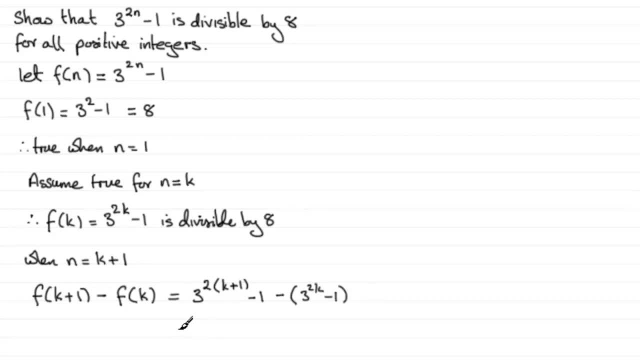 Minus 1.. Now, let's just tidy this up. What we've got here, if we were to expand the brackets, is 3 to the power 2k plus 2. And then we've got minus 1 here and then minus 3 to the power 2k. 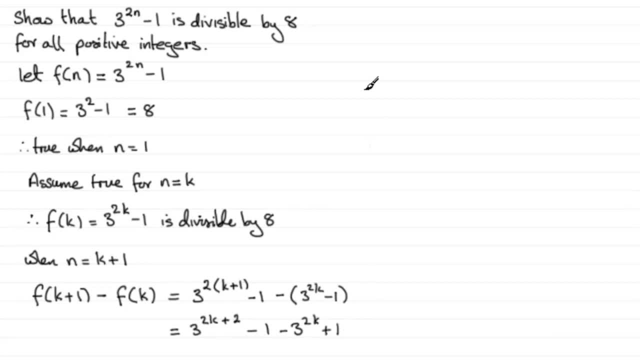 and then plus 1.. And then, if we continue down here, let's just write this out again. We therefore have f of k plus 1 minus f of k equals Right now the minus 1 and the 1. that cancels out. but here, when we're adding the powers, its the same. 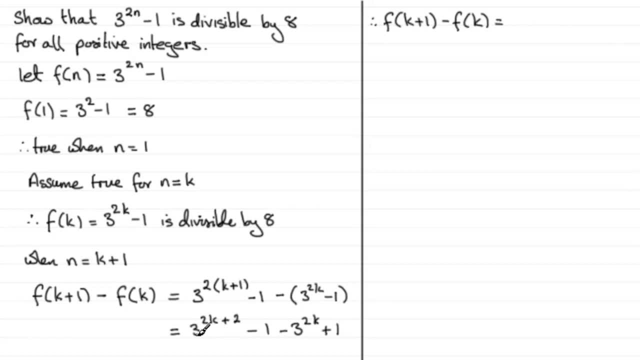 as doing: 3 squared multiplied by 3 to the power 2k, 3 squared, then multiplied by 3 to the power 2k, the power 2k, and then we've got this term here- minus 3 to the power 2k. well, 3 squared is 9. 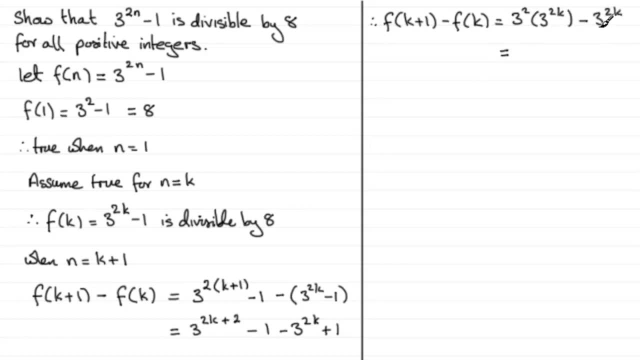 so we've got 9- lots of 3 to the 2k minus 1 lot of 3 to the 2k. so in other words, we've got 8- lots of 3 to the power 2k. now this stage- we always add the f of k to both sides, leaving us with f of k plus 1. 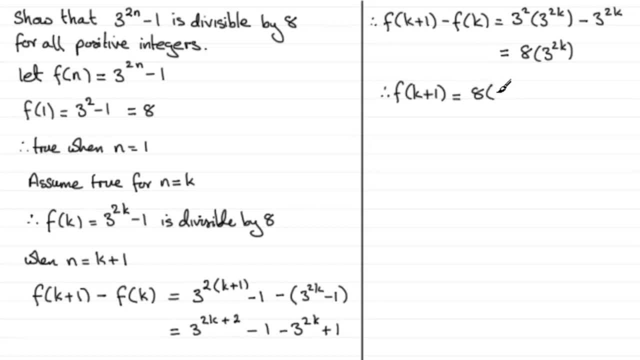 so we've got 8 multiplied by 3 to the power 2k and then plus f of k. now we can see that f of k plus 1 must be divisible by eight, because we've got two terms here. this term, f of k, is divisible by eight. we 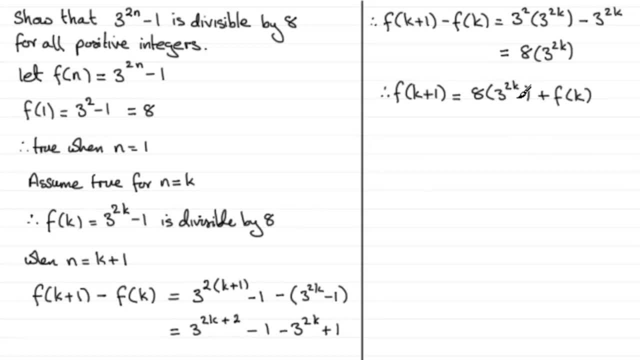 made that assumption and this term here is divisible by eight because you've got three to the power: two k, k being an integer means that this is an integer and it's multiplied by eight, so this term is divisible by eight. we've now got both terms divisible by eight, so f of k plus one. 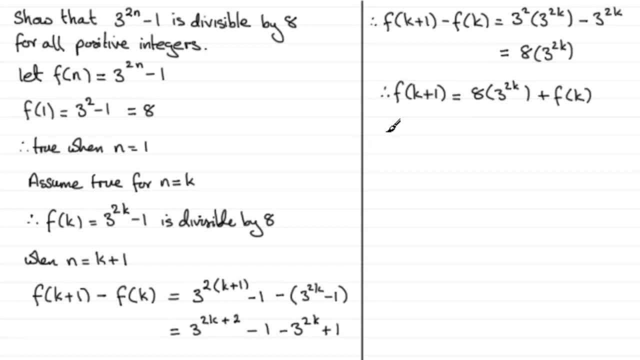 must be divisible by eight. so we can say that since both terms, okay- are divisible by eight, just write that in divisible by eight. okay, then f of k plus one must be divisible by eight. right now we can see that, if it's true, okay, if true, for n equals some value k, then we've just proved that it's true: for n equals k plus one. 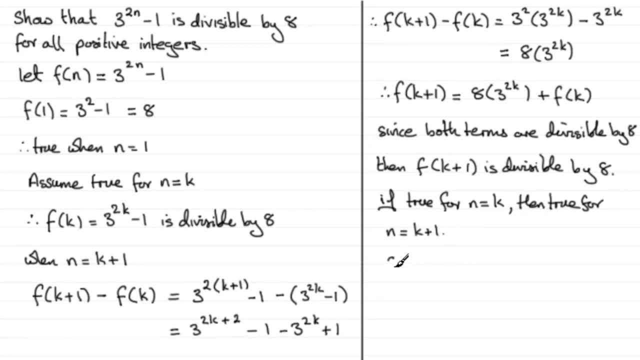 by n equals one, and so we now know that it's true. i can write here: since true for n equals one, we prove that in the first instance up here, then it must be true for n equals 2, and if true for n equals 2, it must be true for three, and if it's true three, four and so on. so in fact it's therefore.